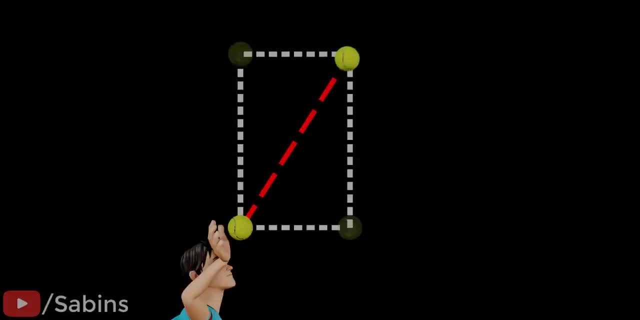 Its complete motion will be as shown. Since the horizontal component of velocity does not change with time, with an equal time interval, the ball will travel the same distance horizontally. However, the vertical component of velocity has been reduced due to the effect of gravity. 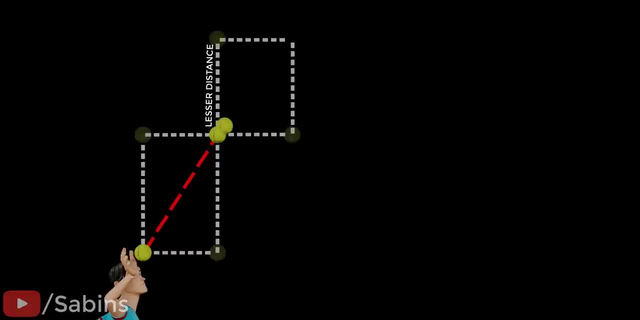 Thus the distance traveled vertically in this trajectory is not the same as the horizontal component. Therefore the horizontal component of velocity does not change with time. With the vertical component of velocity, it will not shift until the horizontal component of velocity is reduced. Thus its' total vertical content is reduced. 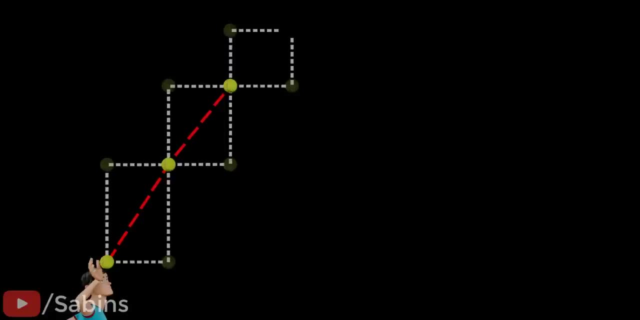 Just continue this logic for few more intervals. You can clearly see the object is taking a curved path As the vertical velocity keeps on decreasing as the ball travels up, the point where the vertical velocity becomes zero will be the maximum height it can achieve. 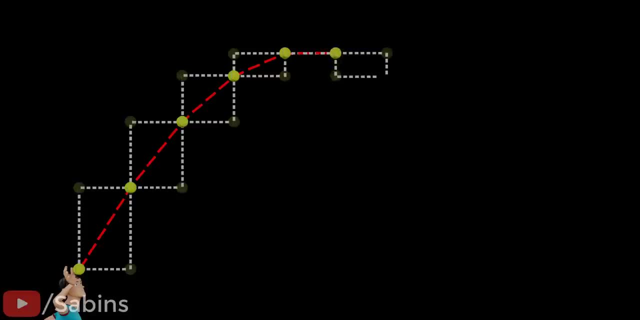 After this point, the vertical velocity will become negative and the object will start its descent. During the descent, the gravitational force and velocity are in the same direction, so the vertical velocity will keep increasing. This will be the final shape traced by the ball. The shape of this trajectory is known as a parabola. 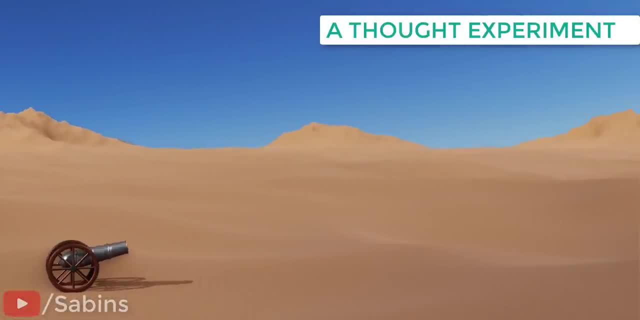 Here's an interesting thought experiment. This cannon is ejecting a ball perfectly vertically. The ball will come back to its initial position, or zero movement in the horizontal direction. Now let's reduce the angle and eject it with the same speed. Now the ball can travel horizontally With a little more angle reduction. 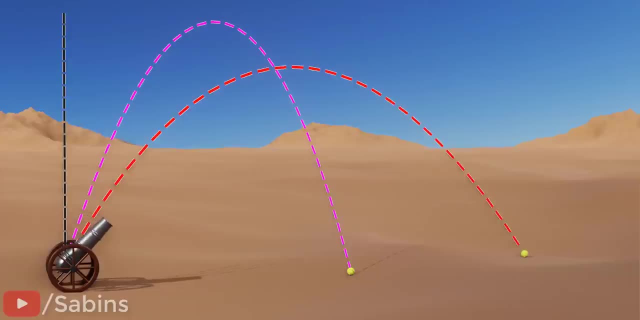 the range increases further. When the cannon's angle is down to 45 degrees, the range becomes even higher. However, if you increase the angle after 45 degrees, the outcome is different. The range actually decreases. The maximum range is at an angle of 45 degrees. Before and after that, the range decreases. 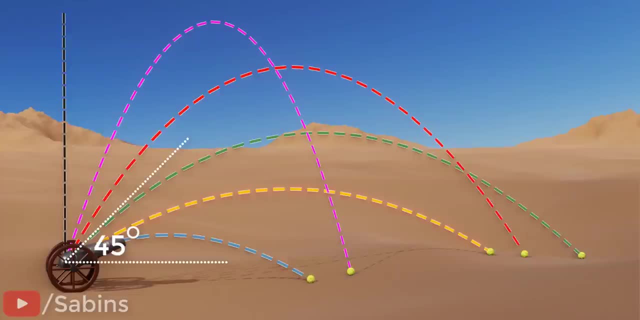 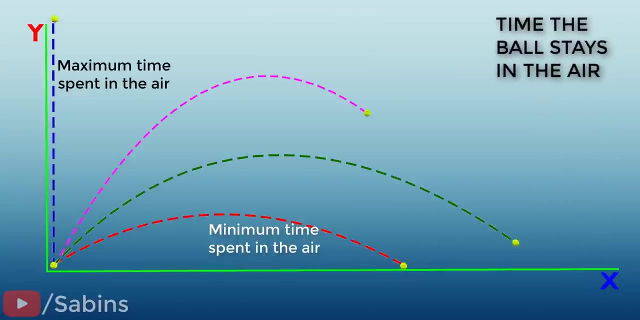 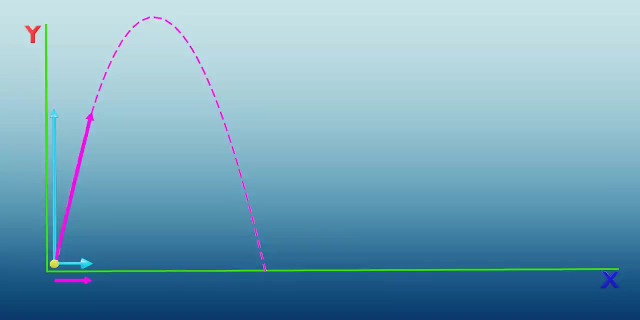 Can you guess the reason behind this? The range of the ball is multiplication of the initial horizontal velocity you have given, multiplied by the time duration it stays in the air. The time the ball spends in the air decreases as you decrease the angle. However, the horizontal velocity keeps on increasing as you reduce the angle. 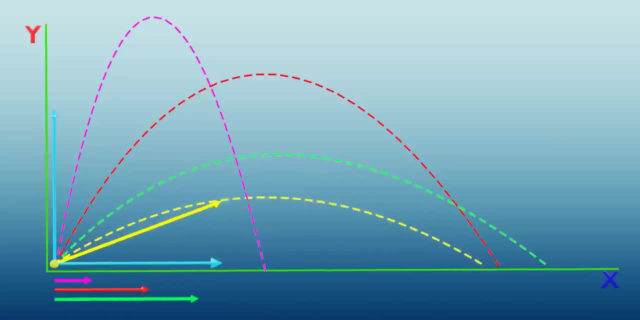 Multiplication of two numbers will be maximum when both the factors have a good value. In this case, the time the ball spends in the air and horizontal velocity has a good value at an angle of 45 degrees. This is why you get maximum range when you throw the ball at 45 degrees. 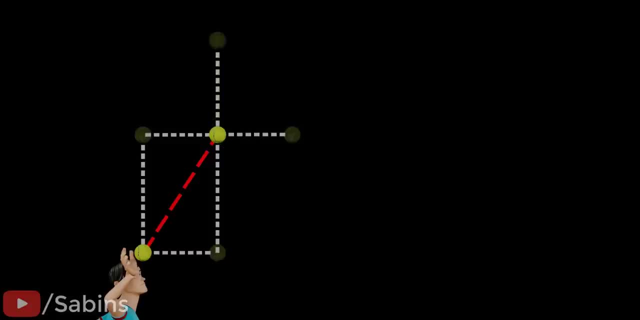 However, the vertical component of velocity has been reduced due to the effect of gravity. Thus, the distance traveled vertically in this situation will not change. Thus, the distance traveled vertically in this situation will not change due to the effect of gravity. Just continue this logic for a few more intervals. 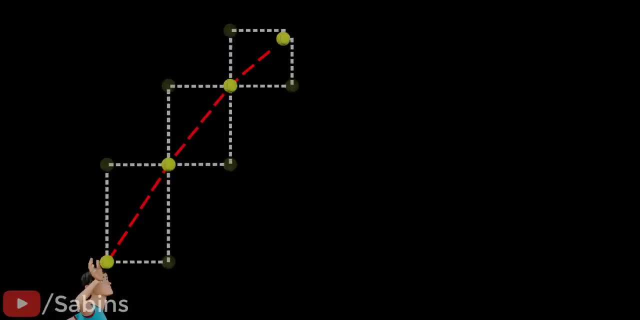 You can clearly see the object is taking a curved path As the vertical velocity keeps on decreasing. as the ball travels up, the point where the vertical velocity becomes zero will be the maximum height it can achieve. After this point, the vertical velocity will become negative. 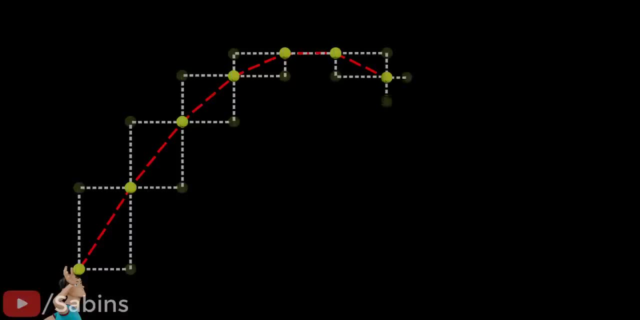 and the object will start its descent. During the descent, the gravitational force and the velocity of the object will change. The force and velocity are in the same direction, so the vertical velocity will keep increasing. This will be the final shape traced by the ball. 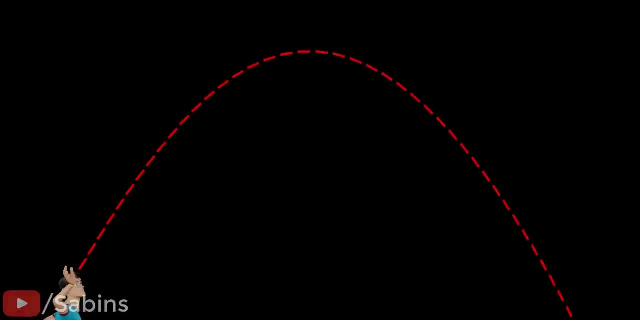 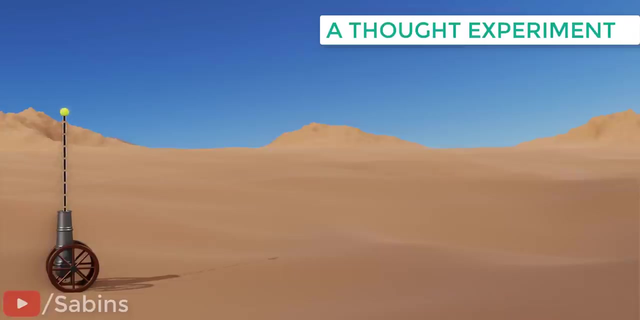 The shape of this trajectory is known as a parabola. Here's an interesting thought experiment. This cannon is ejecting a ball perfectly vertically. The ball will come back to its initial position, or zero movement in the horizontal direction. Now let's reduce the angle and eject it with the same speed. 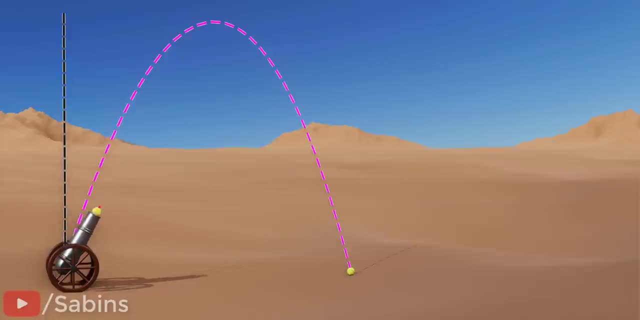 Now the ball can travel vertically. Now the ball can travel horizontally. With a little more angle reduction, the range increases further. When the cannon's angle is down to 45 degrees, the range becomes even higher. However, if you increase the angle after 45 degrees, the outcome is different. 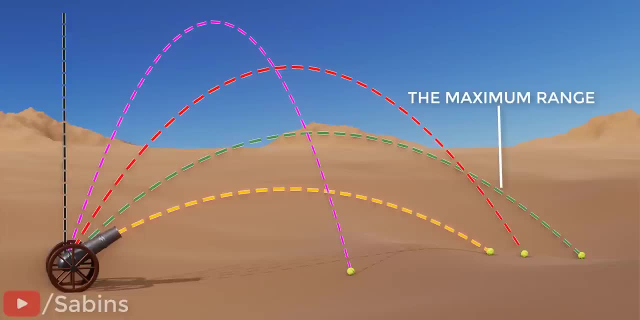 The range actually decreases. The maximum range is at an angle of 45 degrees. Before and after that, the range decreases. Can you guess the reason behind this? The range of the ball is multiplication. The range of the ball is the ratio of the initial horizontal velocity you have given. 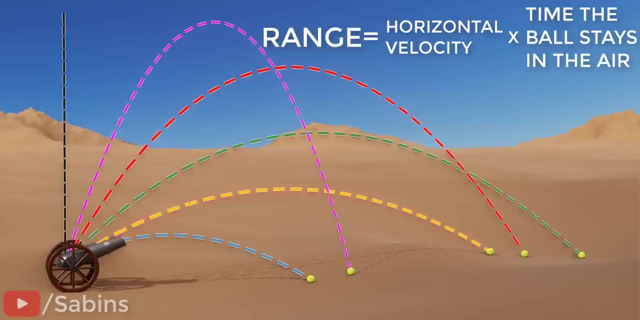 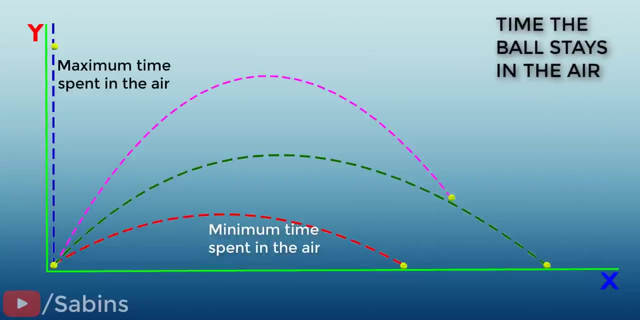 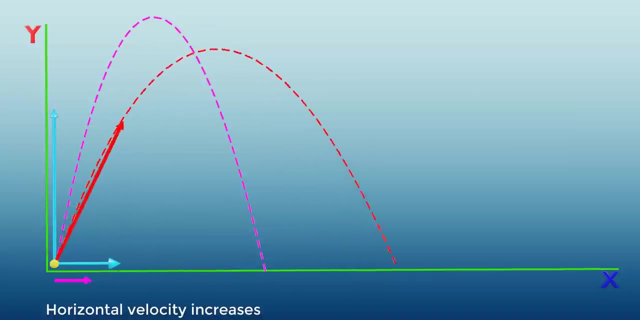 multiplied by the time duration it stays in the air. The time the ball spends in the air decreases as you decrease the angle. However, the horizontal velocity keeps on increasing as you reduce the angle. Multiplication of two numbers will be maximum when both the factors have a good value. 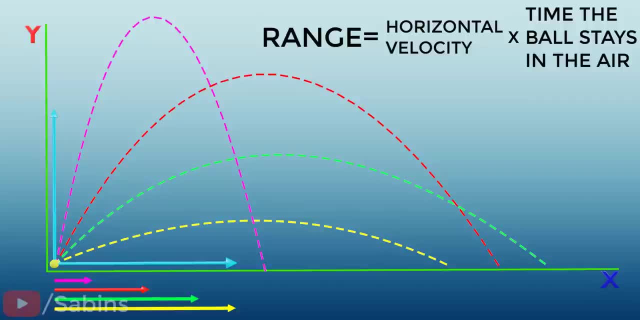 In this case, the time the ball spent in the air is a maximum. The time the ball spent in the air and horizontal velocity has a good value at the angle of 45 degrees. This is why you get maximum range when you throw the ball at 45 degrees.